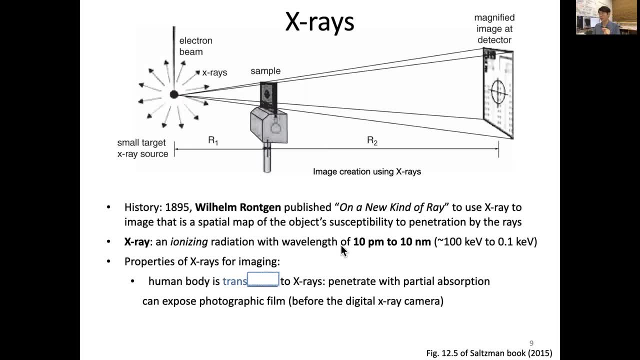 size of a hydrogen atom, And this is a pretty long wavelength, And we call this wavelength a嚼 wavelength, which is basically a wavelength, that'sошage, of a hydrogen atom. This is because this wavelength, which is called a wavelength of the hydrogen atom, is quite short, and 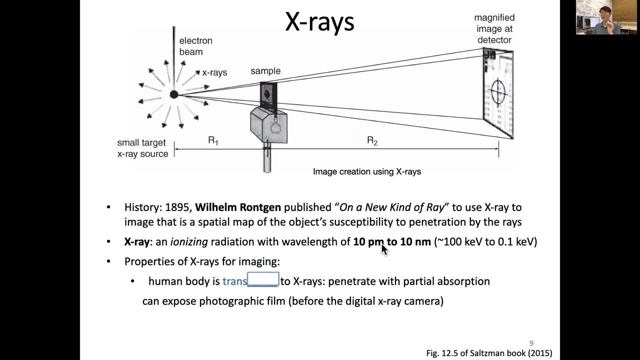 the energy of this photon is pretty high, So powerful. So the wavelength is only about ten picometer to 10 nanometer. Remember 1 Å is the size of a hydrogen atom. So this is pretty, pretty short wavelength, meaning that the energy is high. So the energy is. 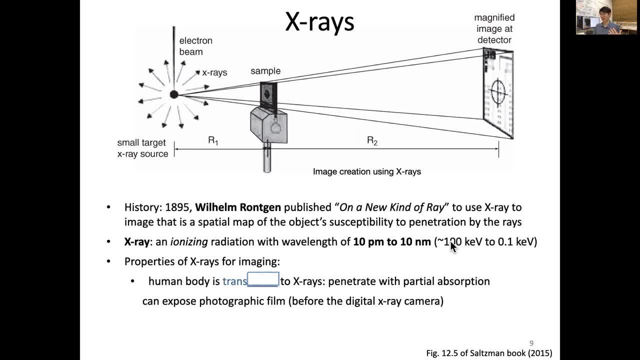 almost about 100 kilovolts, which is a very short wavelength. So this is a pretty pretty electron volt to about 0.1 kilo electron volt. so this can hit the target and actually ionize, which means the it can eject electron, the valence electron out. 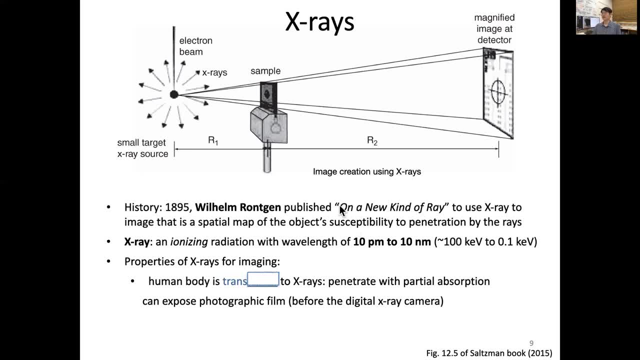 of the, an atom. so, however, this is a can be useful medically. so you see, electron beam shoots target which you will send out x-rays outside, and this is so powerful that through the sample it penetrates, through the sample you can see. it doesn't even bend or diffract. and so well if you have a film on somewhere. 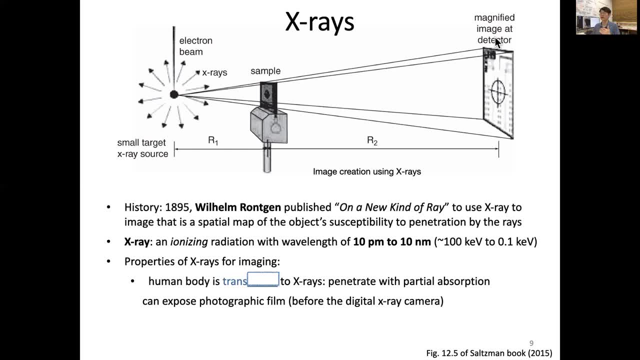 in distance are two, then you can see a magnified images. so between this r1- r2, you can see our one with respect to r1. you can see. between this r1- r2, you can see r1 with respect to r1- r2, you can see. 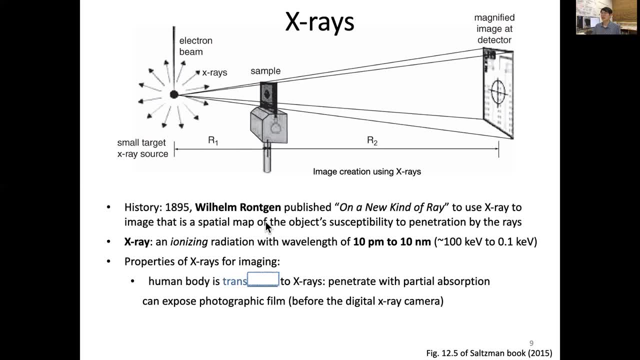 r1 with respect to r1 and you can see r2. you can see r1 with respect to r1 and plus R2 will be magnified. So the properties of x-ray for imaging is because our human body is translucent to x-ray. 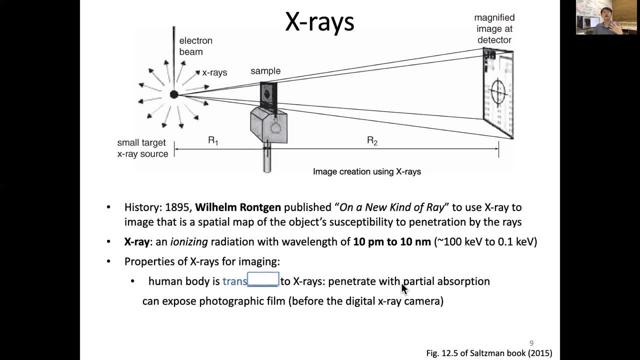 which means the x-ray can penetrate, with a partial absorption which can expose photographic film in the past And now we have digital x-ray camera. So translucent means it's in between transparent and opaque, So that gives us a core ways of looking first time. 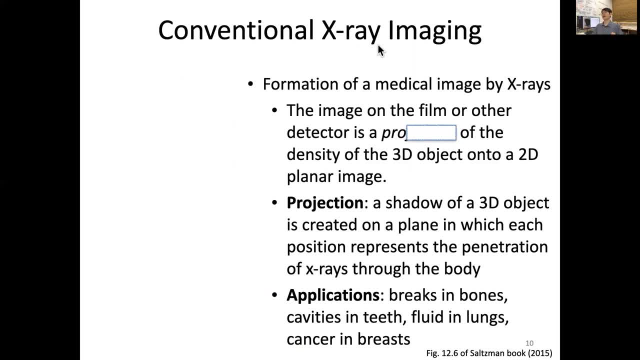 through inside the body. So conventional x-ray imaging is a formation of medical imaging by x-rays. So let me just explain conventional x-ray imaging. As you see, there is an x-ray source or tube. There's an x-ray source or tube. 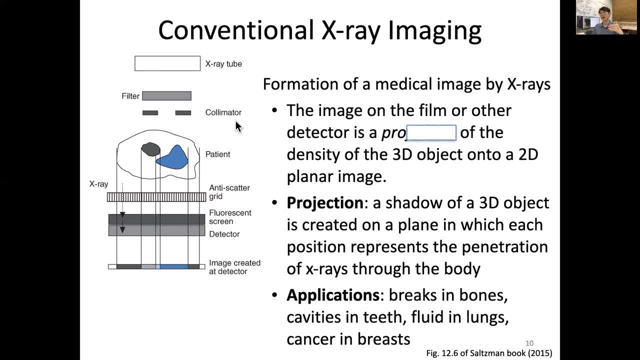 There's an x-ray coming out, There are filters and collimator making the x-ray direction into a parallel. in this particular case, Then this is, let's say, a patient body. Let's say, this black one represents a bone and this color represents some other organ. 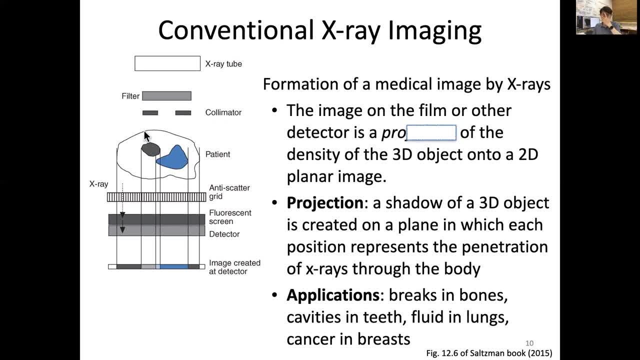 And that x-ray is penetrating because it's high energy photon that it actually represents. Actually, we put as a ray, which means it won't bend, It, just go straight, And we have an anti-scatter grid which blocks the scattered x-ray. 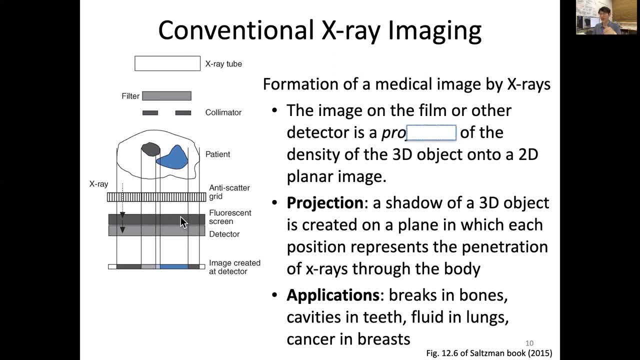 So it passes through and it hits a fluorescent screen And that is a detector. So we can use either film or this fluorescent screen or we can image it using image created at the detector. So you can see that x-ray passing through this part will be different contrast. 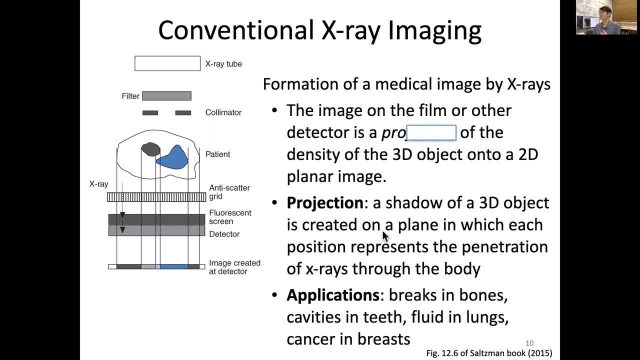 because it has been observed much okay. So the image on the film or other detector is a projection of the density map of the 3D object. But we are looking only 2D planar or 2D projection And the projection is a shadow of a 3D object. 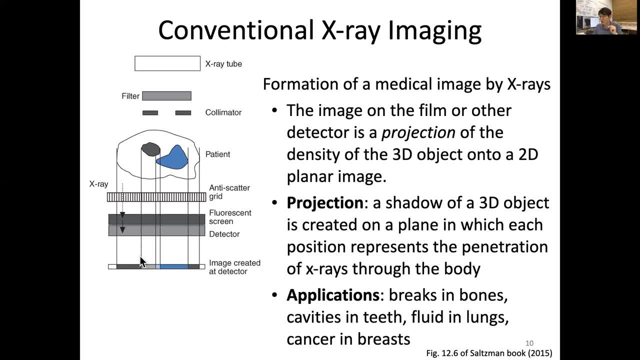 It's created on a plane in which each position represents the penetration of x-ray through the body, the full penetration, And this simple two dimensional projection has been very useful that the applications include breaks in bones, cavities in teeth, fluid in lungs and even cancer in the breast. 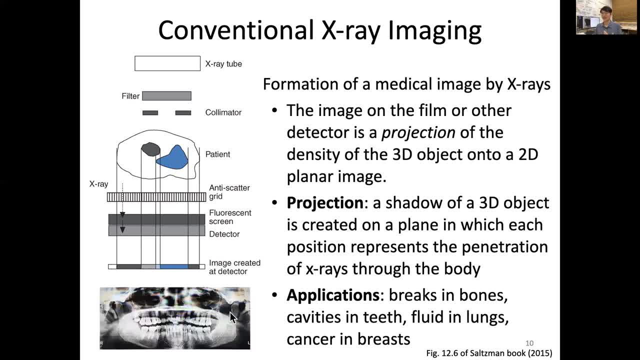 So I brought one example of my teeth from dental x-ray. So you know, with this this is the x-ray source- rotate through my face and it takes this x-ray figures And that, particularly the dentist, showed me that I have this gap between this right side of my teeth. 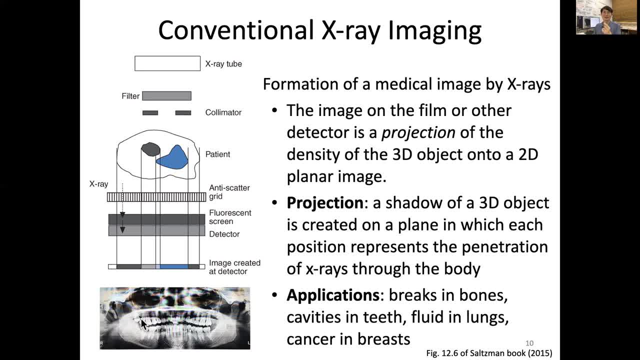 And this happens to be the place whenever I ate some meal and there are like foods and beverages will be kicking in inside. So after this, I understand the importance of flossing After meal, because I realized this part is always many times it has a problem. 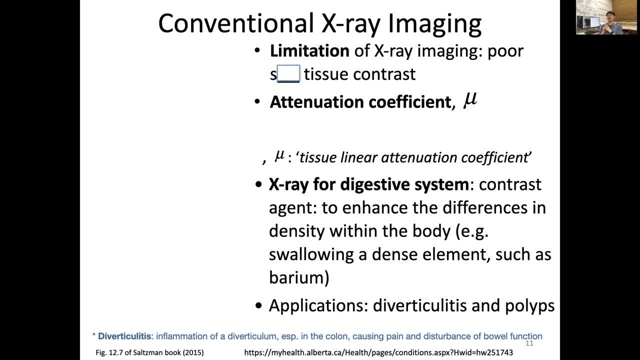 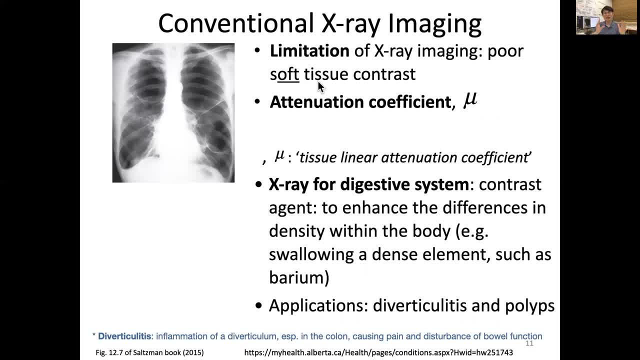 Soft tissue contrast. So, because the contrast mechanism is the absorption of the x-ray, where which is a bone is the most easily absorbing the x-ray, So that we are based on this attenuation and we can have attenuation coefficient for each of this tissue. 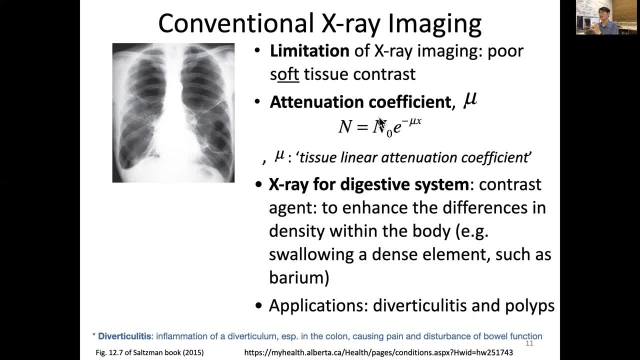 So that original signal of N0. after, through this x-ray, this x amount of tissue that will be reduced by exponential decay with N, So that mu is called tissue linear attenuation coefficient And you can see the unit will be one over length. So the example of x-ray for digestive system. 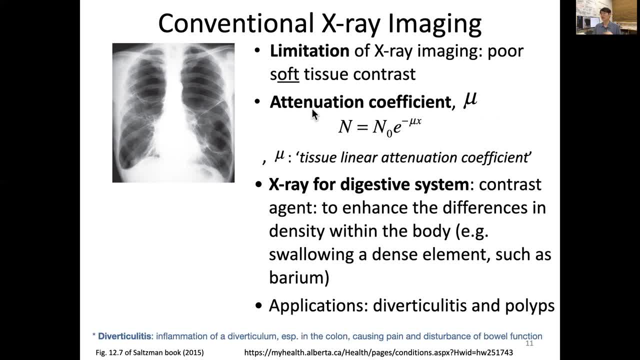 and sometimes because of this poor soft tissue contrast, we use a external contrast agent to enhance the differences in density within the body, For example swallowing a dense elements such as a barium, and then that can show the internal gut, So for example, diverticulitis. 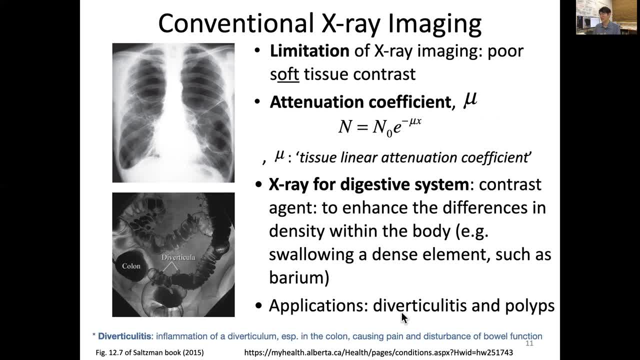 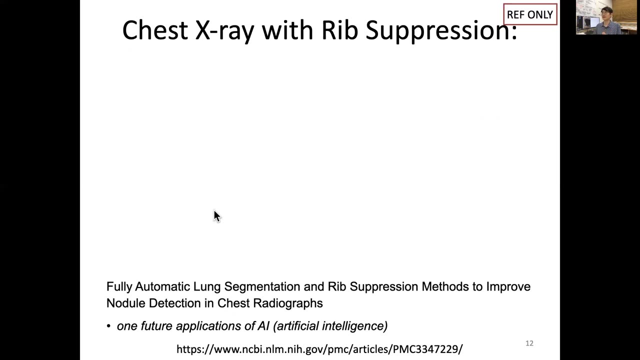 which is a lightest means. inflammation in the diverticulum And sometimes polyp, which is cancer, pre-cancer inside colon can be detected by using this help of contrast enhanced x-ray. So I just bring some light Nowadays. what's cool about this x-ray?